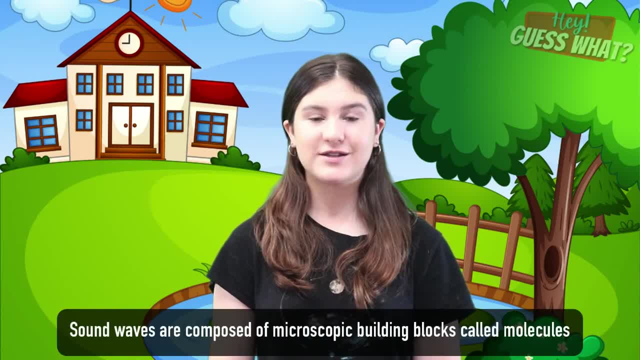 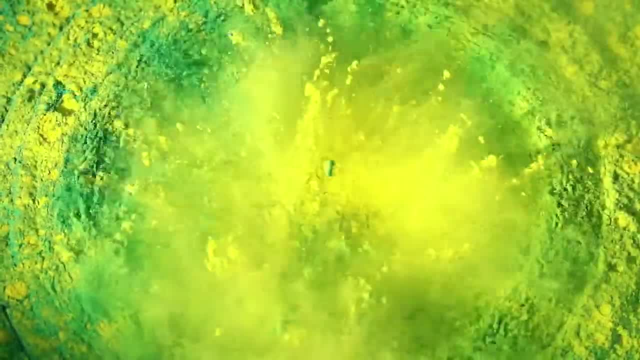 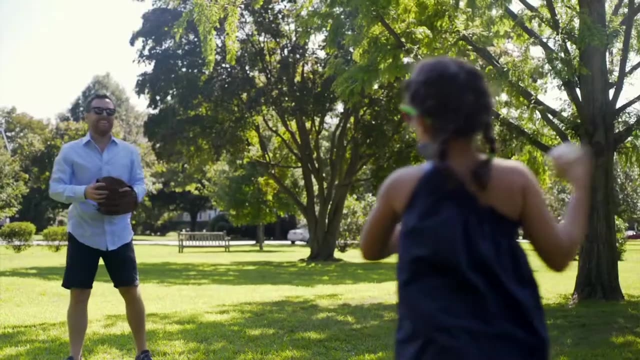 Sound waves are composed of microscopic building blocks called molecules. Sound waves travel back and forth through solids, liquids and even gases to get to another location. Think of it like throwing a ball back and forth to play catch. Sound waves also travel back and forth, just like the ball. 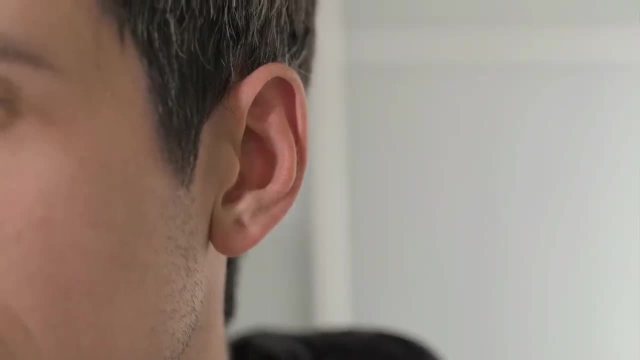 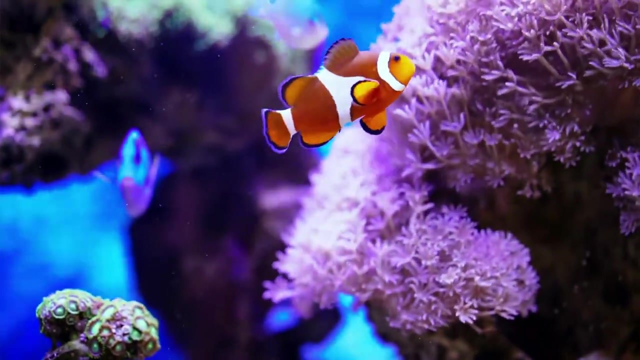 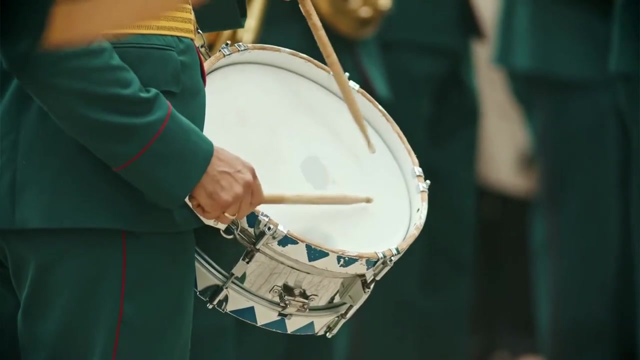 When you play catch with someone else. Sound waves are how you can hear sounds that are close to you, happening outside or even underwater. Have you ever been to a concert or a football game or a marching band? Well, you may have felt vibrating energy from these sound waves while you were there. 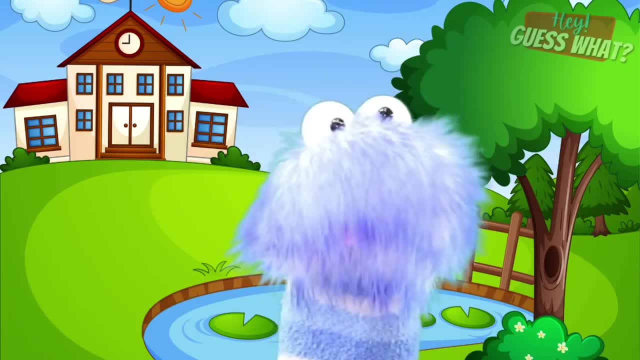 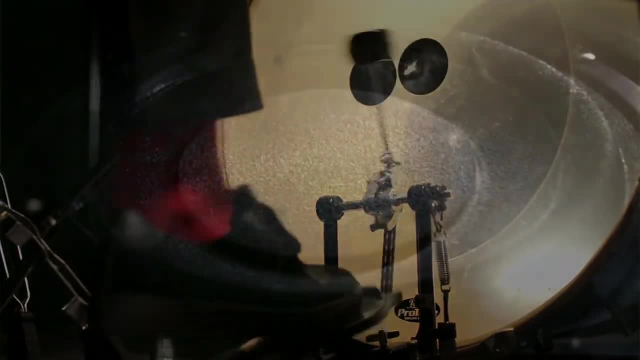 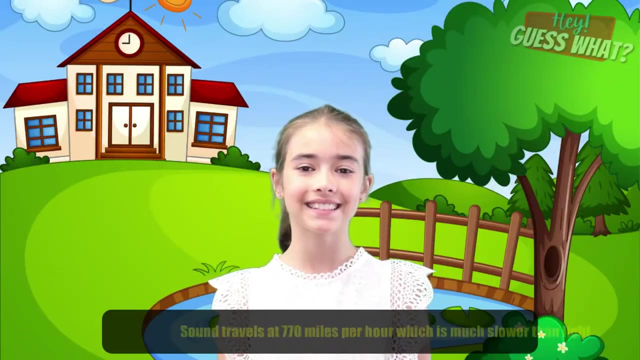 in your feet or sometimes even in your chest. Hey, guess what? That's actually right, Gus. Some instruments create sound vibrations so powerful that you actually do feel the vibrations in your chest. Sound travels at 770 miles per hour, which is much slower than light. 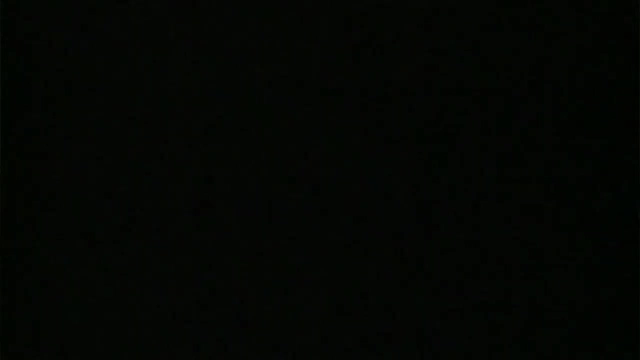 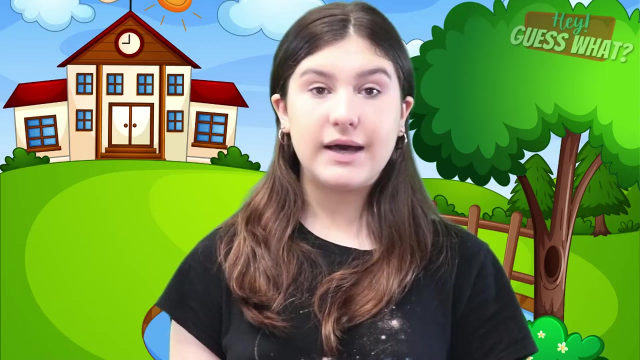 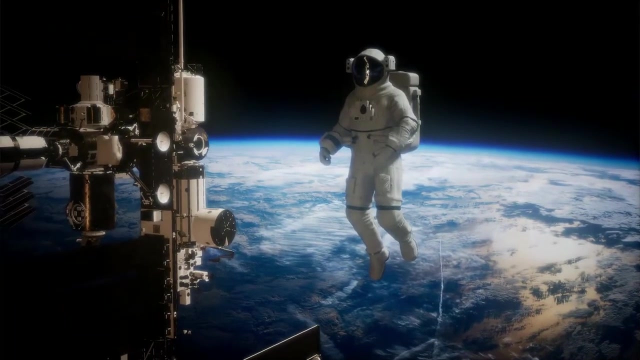 Sometimes you hear things after you see them, For instance, like flashes of lightning before you hear the thunder. But sound waves cannot travel through a vacuum, which is a place with nothing in it, And that is why astronauts cannot talk to each other in space. 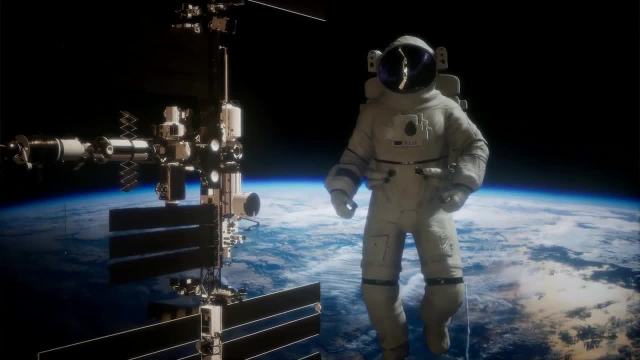 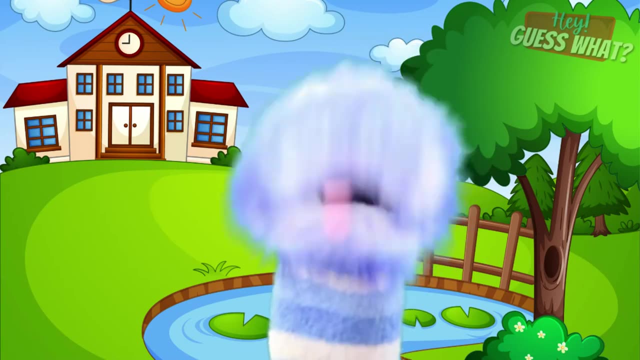 and they need a radio to hear each other, because in space there is nothing for the sound waves to vibrate off of. Hey, guess what? Did you know that sound travels through water quicker than through the air, And everyone else knows this by heart. 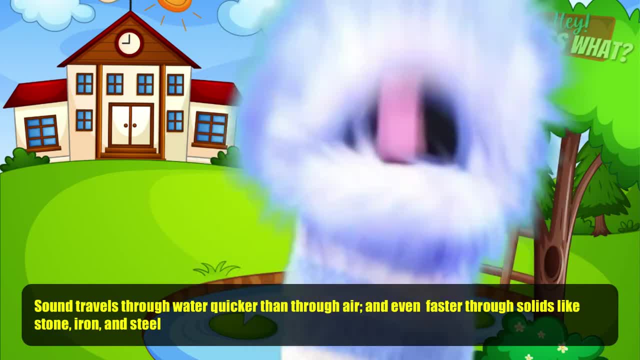 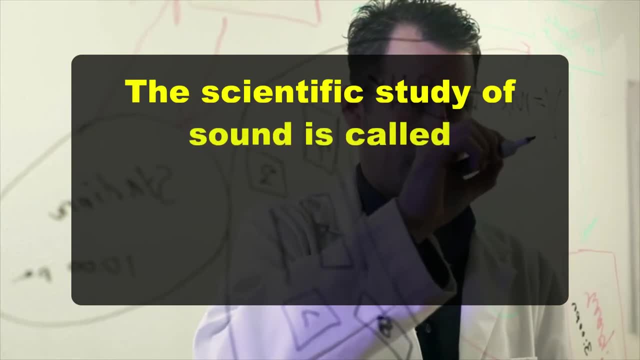 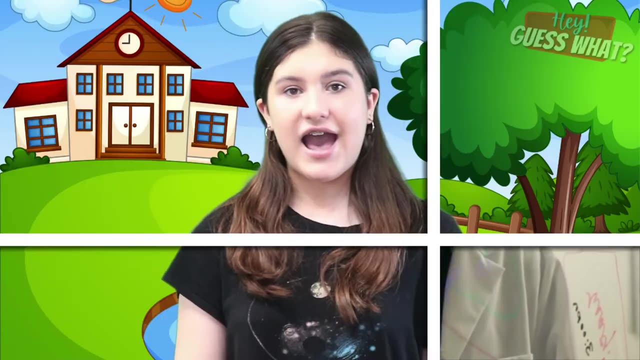 And even faster through solids like stone, iron and steel. Whoa, Hey, guess what? The scientific study of sound is called acoustics and we measure how loud sounds are in decibels. How loud a sound is depends on sound intensity. 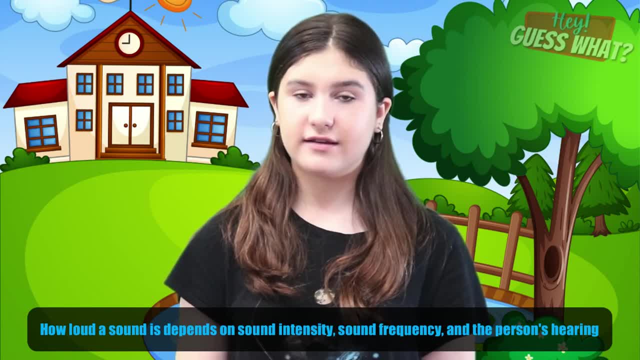 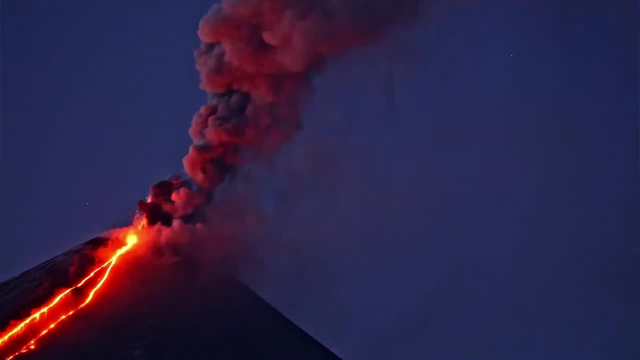 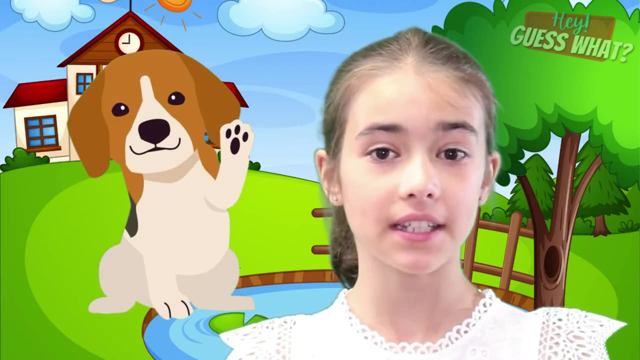 sound frequency and the person's hearing. The loudest natural sound on our planet Earth is a volcanic eruption. Dogs hear sounds at a higher frequency than humans. This allows them to hear sounds that we can't, And sound is different than noise.